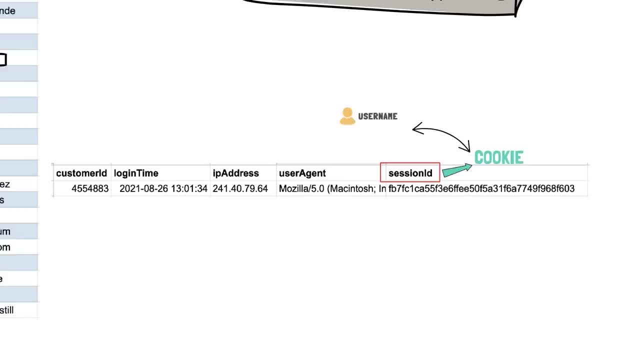 ID in the form of a cookie. In other words, you have exchanged your username and password for this cookie containing the session ID. The session ID is just a unique identifier for your logging session and it is randomly generated. The concept is similar to giving 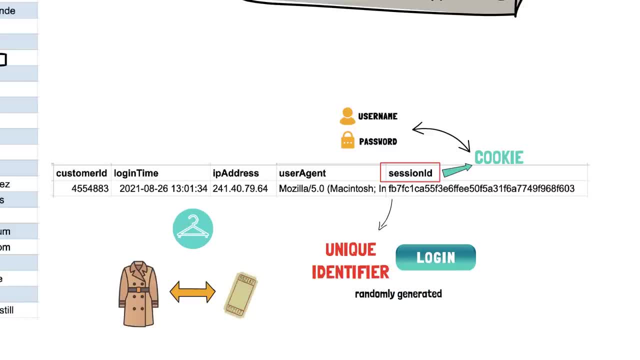 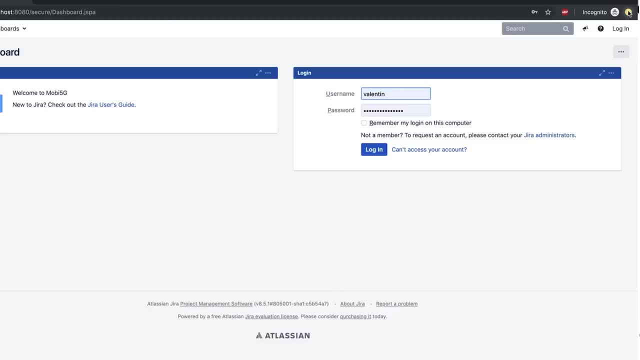 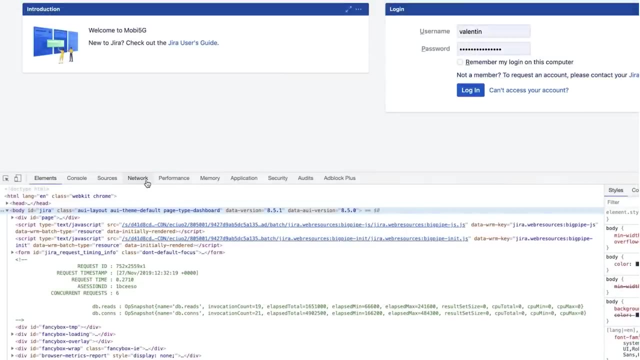 your code at the cloakroom and receiving a ticket with a number. I have explained the basics around cookies in another tutorial, which I will link in the description. You can check this logging process for yourself on almost any website to better understand it. In Google Chrome or any other browser, you can open the developer's 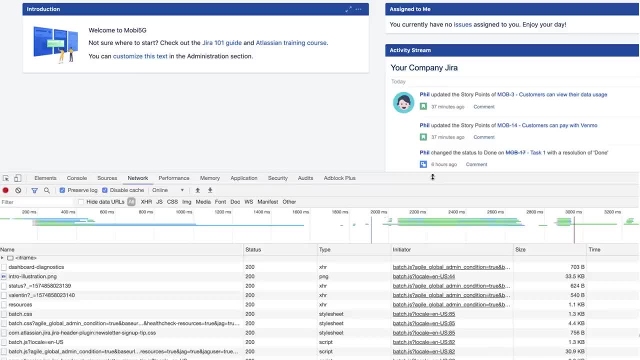 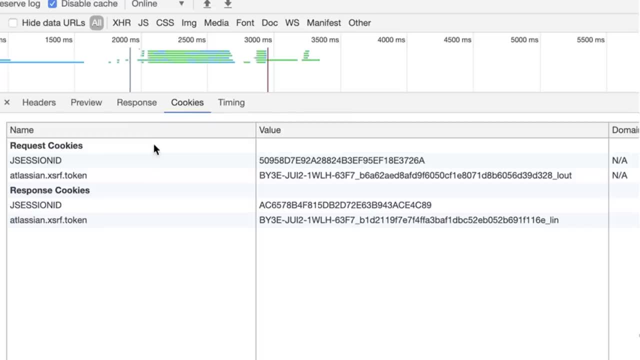 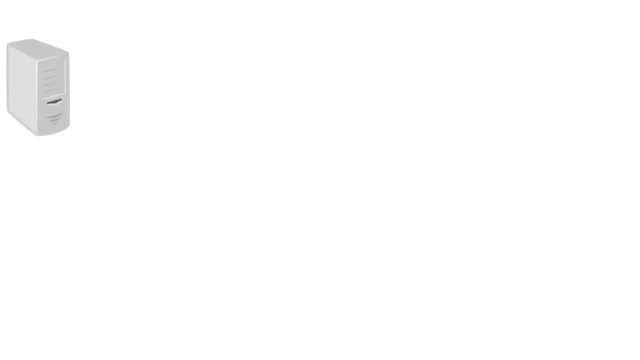 tools and inspect your network traffic. For example, here I have sent my username and password and received a cookie with this session ID. The content of the cookie is the same as the content of the session ID. The content of the cookie is secret and other websites cannot read it, So the server will store the 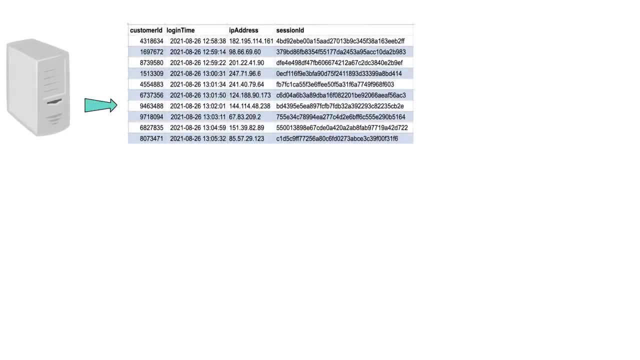 session information in the database and you will only have the session ID in a cookie which is stored on your computer's file system. Next time you request another page, your browser will automatically send the cookie containing your session ID, which the server will check. 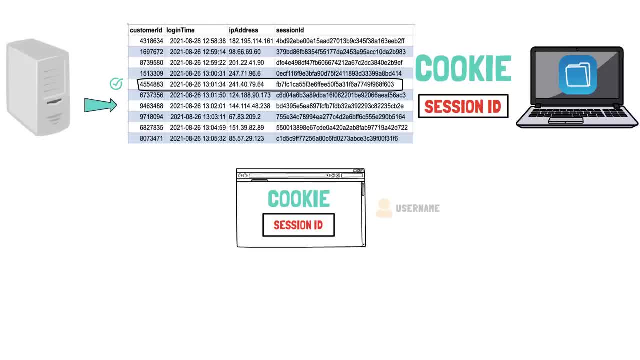 to see if it is still valid. It is essential to notice that the second time, your username and password are no longer required in order to uniquely identify you. If you log out, your log in session will be invalidated in the database, but also the server will instruct. 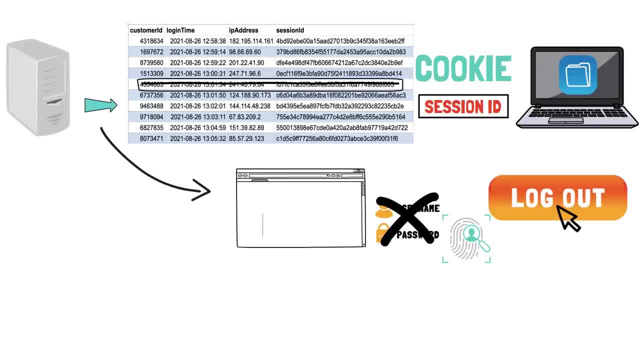 the browser to delete the cookie containing the session ID. Even so, if the session on the server expires, the cookie becomes worthless. Your session will expire. if you are inactive for some time, The bank's server will keep the session active. As long as the cookie remains inactive, the session will be valid. 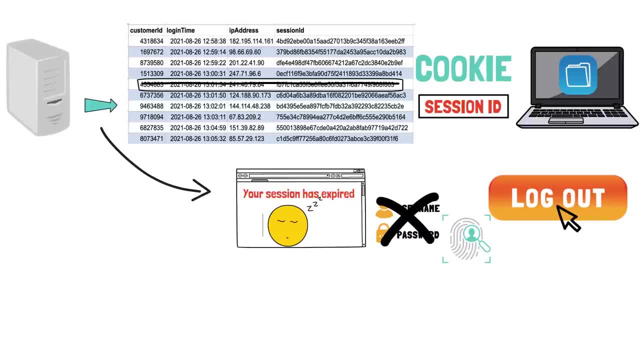 The bank will include your message and password when it is not used and the user will get long as you keep interacting with the server. If, for some time, you are inactive and you want to visit a new page, the server will notice this period of inactivity and will prompt you to. 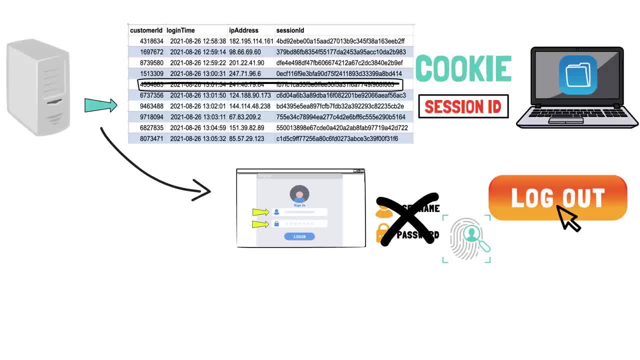 provide your username and password again as a security measure. Some websites, like Facebook, for example, may create a long-lived session, which means that you will rarely need to enter your login credentials. However, your bank may use a very short-lived session, commonly five. 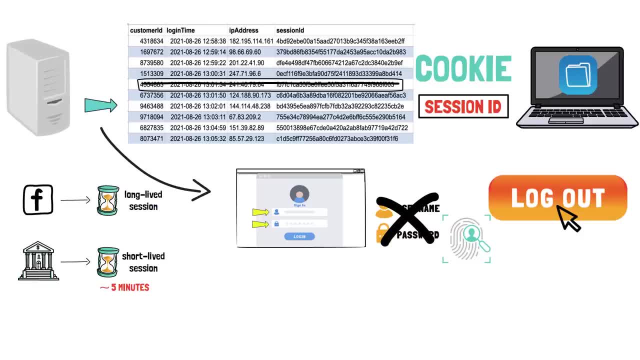 minutes or less. If you are inactive for five minutes, you need to log in again. The concept of a cookie can be hard to grasp. Let me make an analogy. Think about a cookie like your gym membership card. It stores your member ID on it and when you scan it at the entry, it checks if 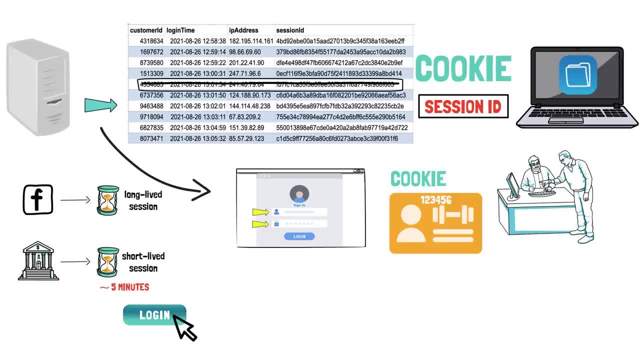 your membership is still valid and lets you in. Again, as with your gym card, a cookie with a session ID only works with a specific website. You cannot use your gym card to enter your office building, for example, And also, if your gym membership expires, your card will become useless. 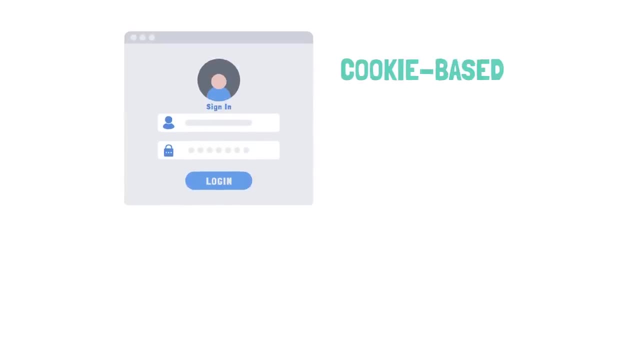 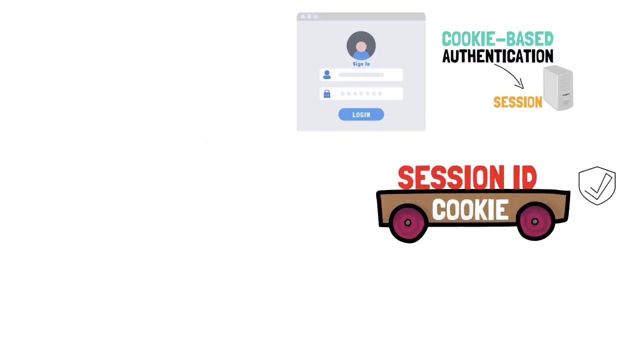 Now let's go back to the login example. This method is called a cookie-based authentication. Accordingly, this authentication used a session on the server to handle this. The cookie is only the medium used to transport the session ID, and it is used because it is convenient. 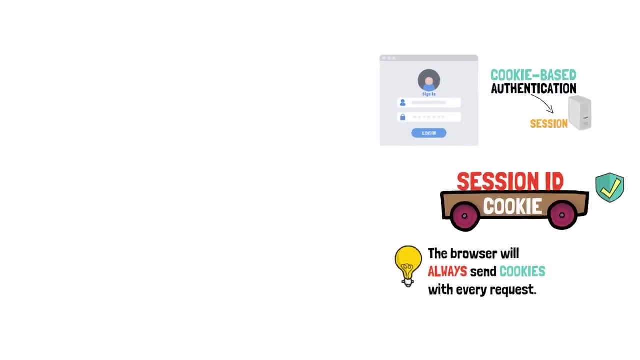 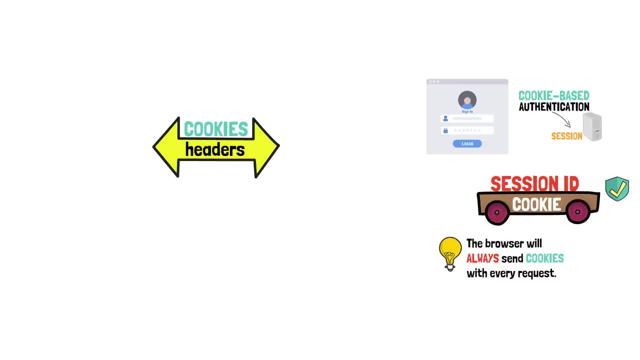 The browser will always send cookies with every request. Technically speaking, cookies are sent using HTTP headers in the messages exchanged between the browser, often referred to as the client, and the server. HTTP is the protocol that ensures that both the browser and the server can understand each other. 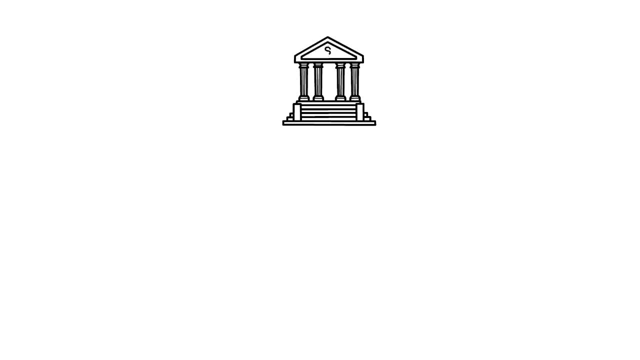 In this case, the bank stores the session information on the server's site and you cannot see the contents of it. This also ensures that you cannot manipulate any information. Let's talk about this real quick. One of the reasons why servers don't store more information. 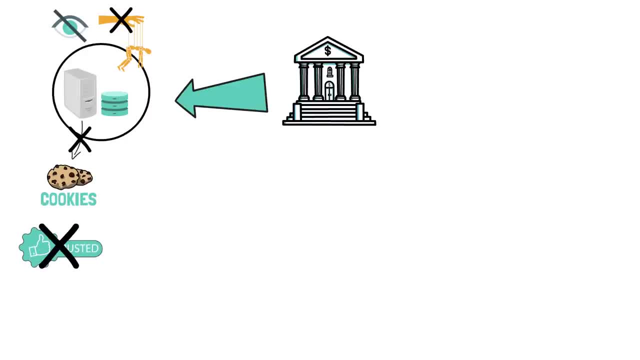 in cookies is that they cannot be trusted as they come from the client. This is a security concern. It is like telling the bank: I have one million dollars in my bank account, just trust me. This is why servers prefer to work with their database, where 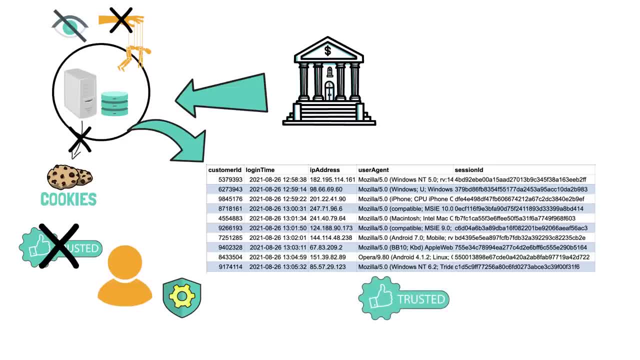 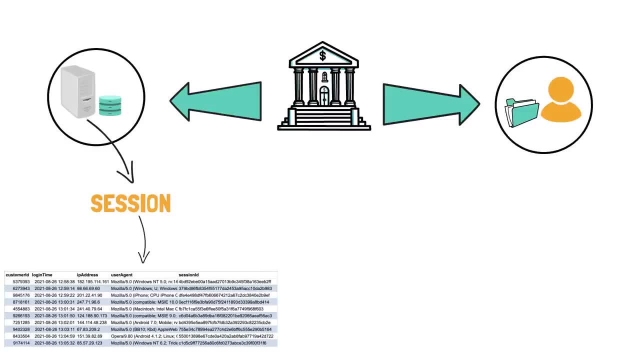 ideally, only valid information exists. So, to recap, the session is generated by the server and will be stored in a database. You, as the client, will only receive the ID of that session, often referred to as the session ID. The session ID is a meaningless, randomly generated and hard to guess sequence of letters. 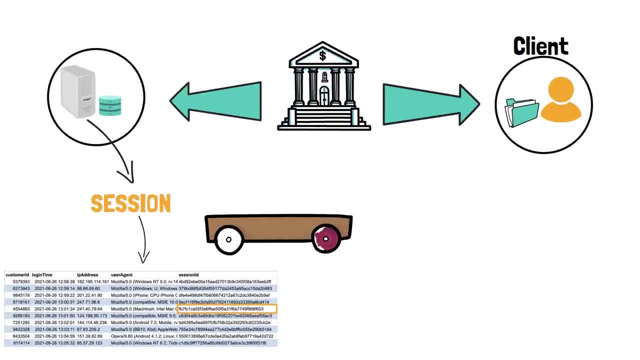 and numbers. Cookies are used as a transport medium for the session ID, as browsers will automatically send any cookies associated with the website. And, finally, as cookies can be modified by the client, the server cannot trust them and always needs to validate them Traditionally, cookie-based authentication. 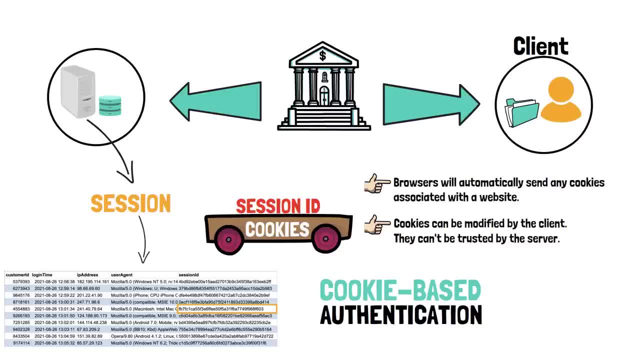 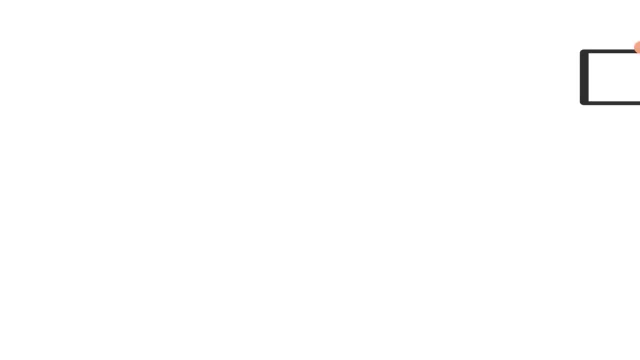 has worked very well for many years, but it is slowly becoming outdated, at least for some use cases. Let's now assume that you want to install an app on your phone which can help you with your finances and keep track of your spending. What you don't want to do is to give your 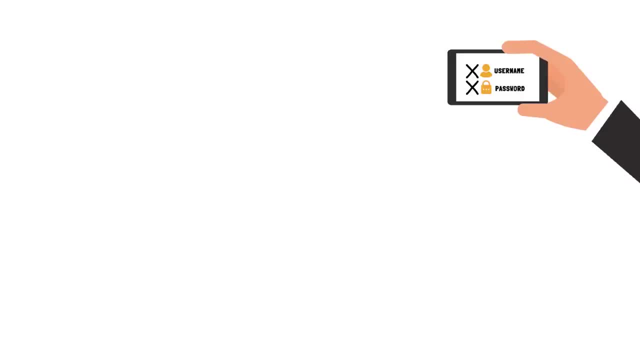 username and password to this app, which is not created nor verified by your bank. In this case, your app will redirect you to your bank. you will enter your username and password and your bank will ask: hey, John, would you like to give this app access to your transactions? 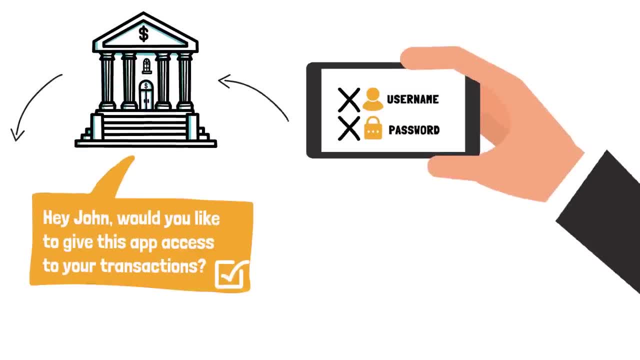 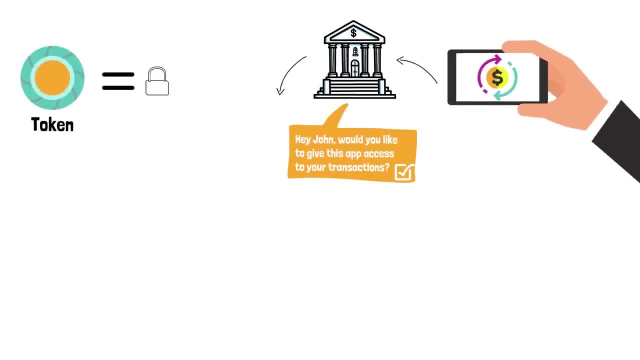 And you will check. yes, and the app will receive a token granting access to your transactions. This token is like a temporary password, if you wish. It is like when you are at a hotel and get a one-day wifi password. However, a token is a bit more than a password Most. 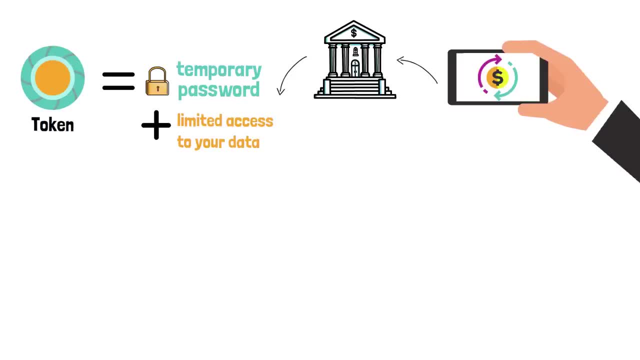 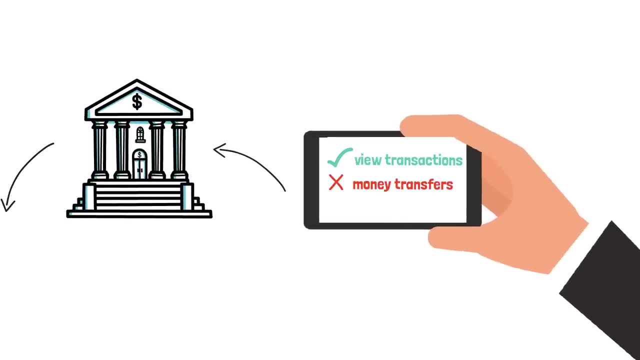 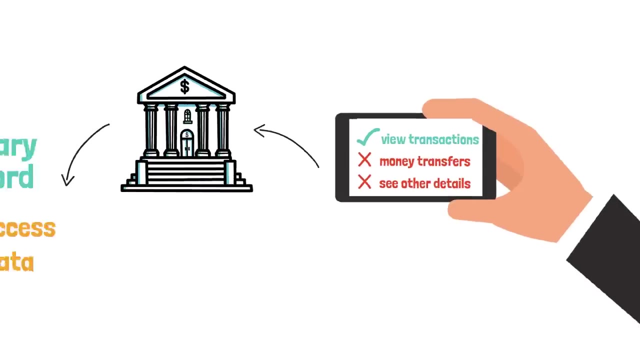 of the time, it will give limited access to your data. In this case, the app will only view transactions. The app will not be allowed to perform money transfers or to see other details. I am sure you have seen a procedure similar to this any time you have used Facebook, Google. 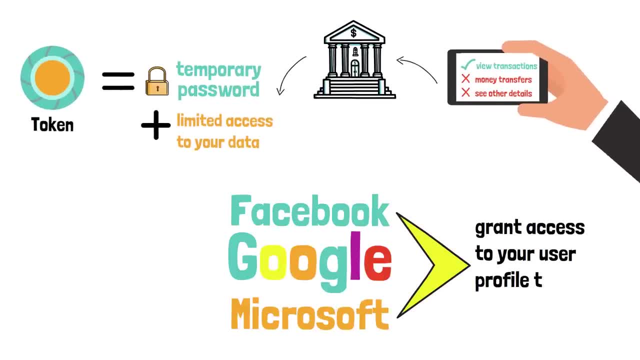 or Microsoft to grant access to your user profile to a third-party website. So in this exchange you never expose your username and password, apart from authenticating with the bank. If you later want, you can easily revoke your bank account. You can also revoke access to your account by invalidating the token which is decoupled. 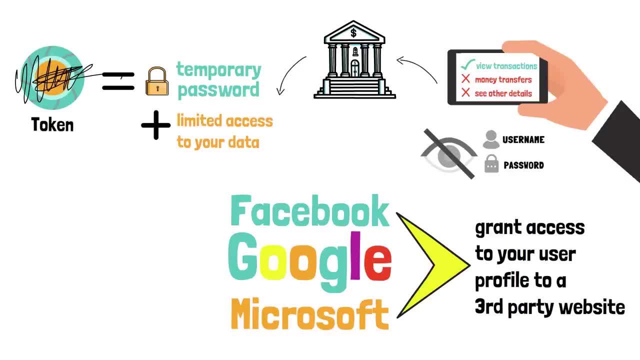 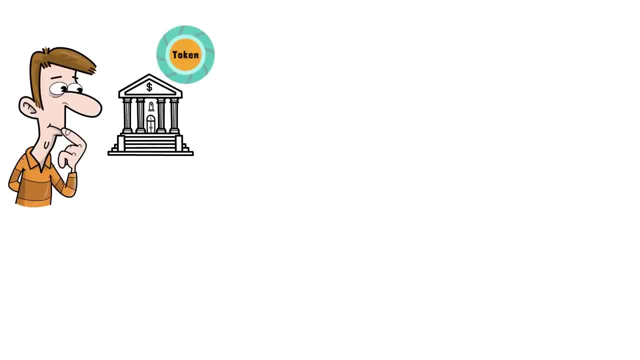 from your account password. One of the most popular protocols used for such scenarios are OAuth, OpenID, but also JWT, which is pronounced JWT. Let's take a look at how a token issued by the bank can look like. Let's use JSON Web. 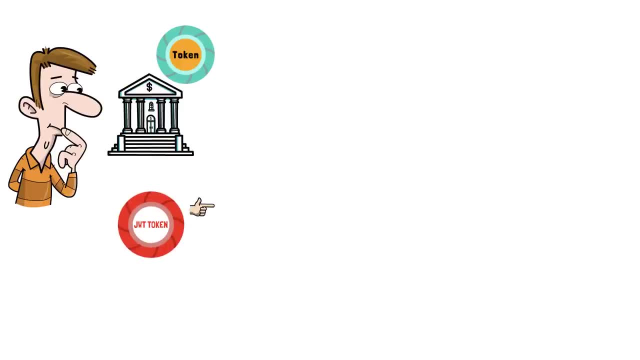 Tokens or JWT tokens. as an example, A JWT token contains the following information: A JWT token contains the following information: A JWT token contains the following information: A JWT token contains more than just a temporary password. The bank may issue a token containing some important information, such as the customer. 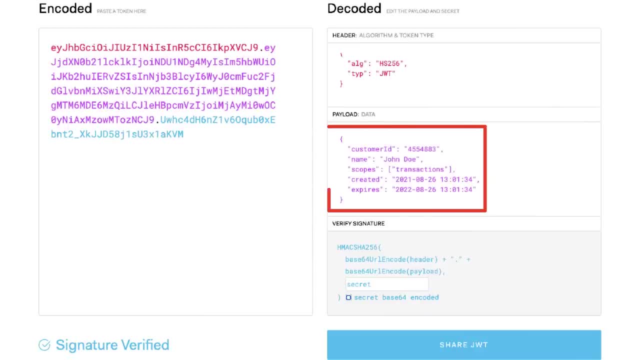 ID, the scope that this token grants, when was the token created and when does it expire? One important aspect to remember is that this information is cryptographically signed. This means that it is easy to verify that the content has not been modified. Tempering. 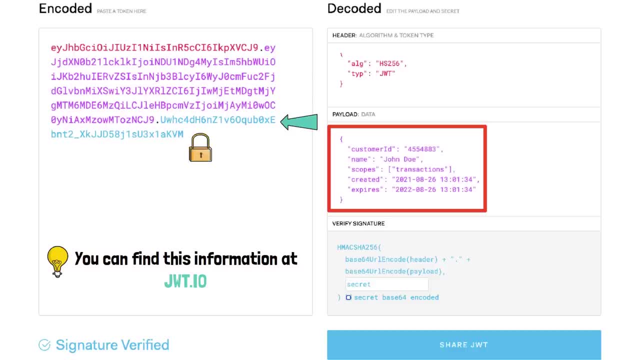 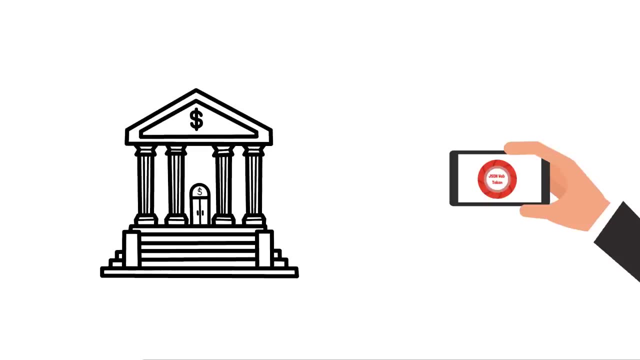 with the content, and generating a new signature is impossible unless you are the bank. The app can use this token to go to the bank and get transaction data or any kind of data that the user has granted access to In this exchange. the app does not know the password of the customer, but it is still. 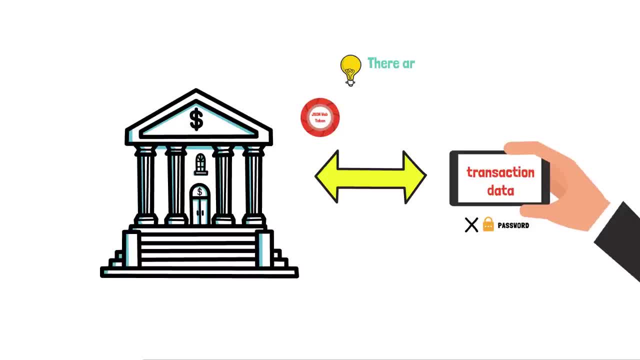 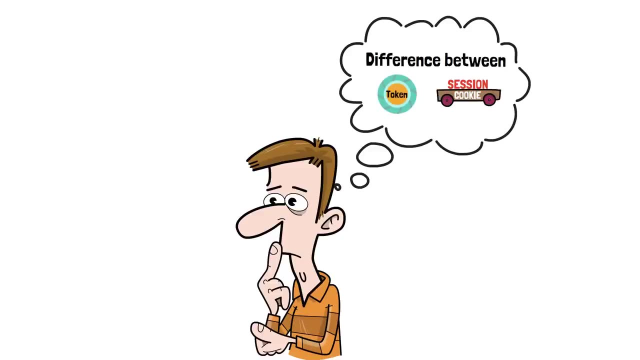 able to retrieve some data. The example I have given is just one use case of many, And there are various ways on how tokens can be deployed and used. So how is this token different from a session stored in a cookie? When using cookies, there are only two parties involved: you and the server. 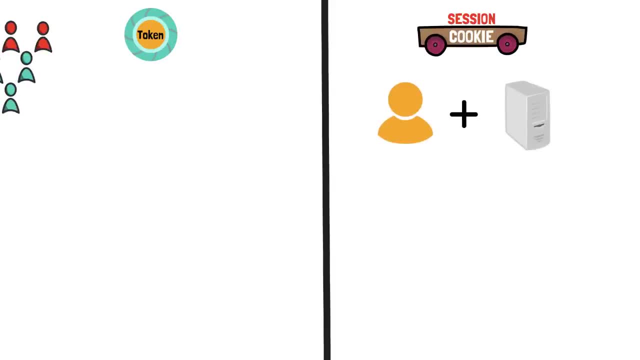 When using tokens, it is essential to notice that the interaction typically involves multiple parties that may not trust each other. So you trust your bank with your bank login details And you trust your bank with your bank login details, But you may not trust this app that you have found in the app store. 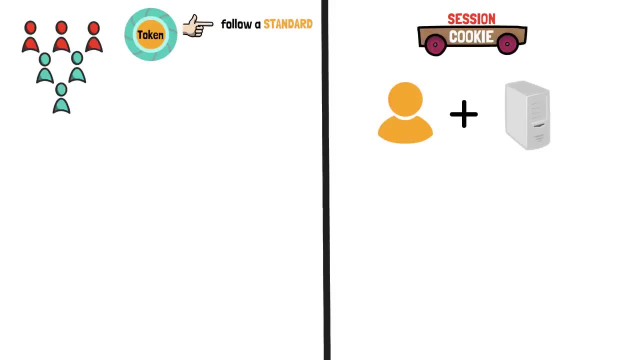 For these reasons, tokens typically follow a standard to ensure interoperability, while sessions are implemented as needed by the server, without necessarily following a standard. Additionally, some tokens tend not to need a session on the server at all. In the case of JAT tokens, the token contains the session information. 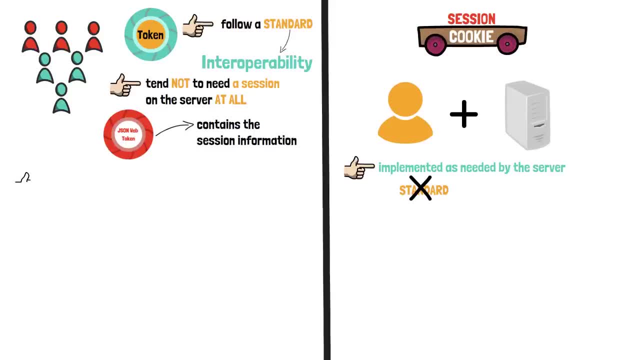 Nevertheless, this is not a rule. Another difference is that the token has a limited lifetime and a new token needs to be generated once it expires. A token can also grant access to only a subset of the data a particular user or entity has.